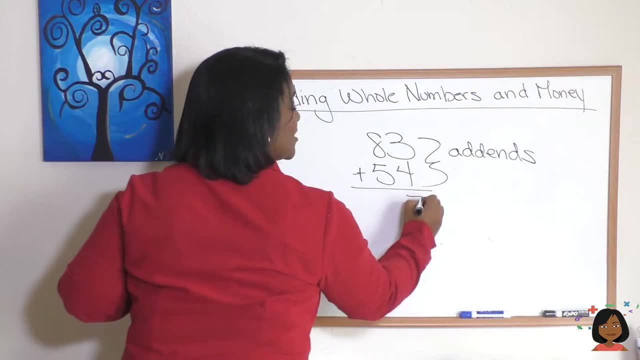 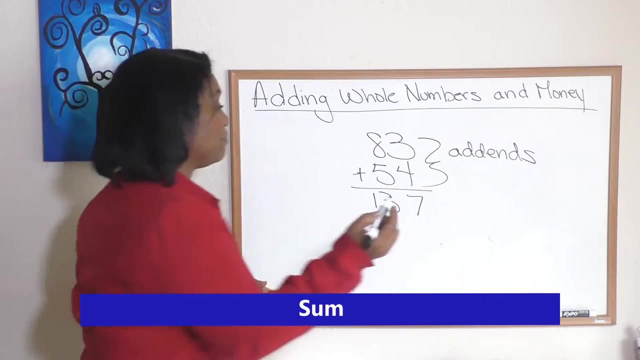 When I add two numbers together so let's go ahead and add them 4 and 3 is 7, 8 and 5 is 13. My number 137 is called the sum. So when we add two numbers together or more than 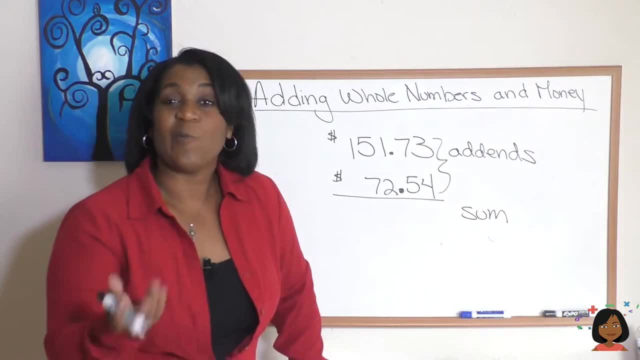 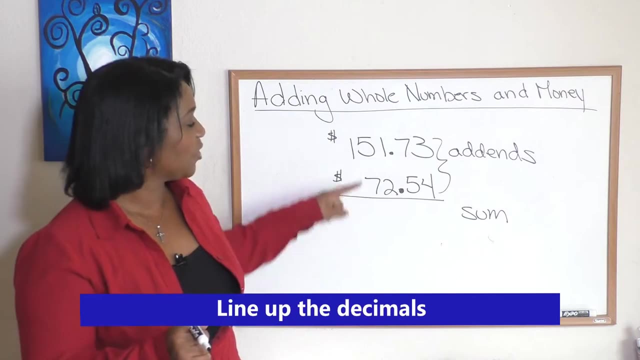 two numbers we call it the sum. Now when we're adding money we still call these our addends and our sum but the one thing that's different about adding money we want to make sure that we always line up our decimal points and then we add. 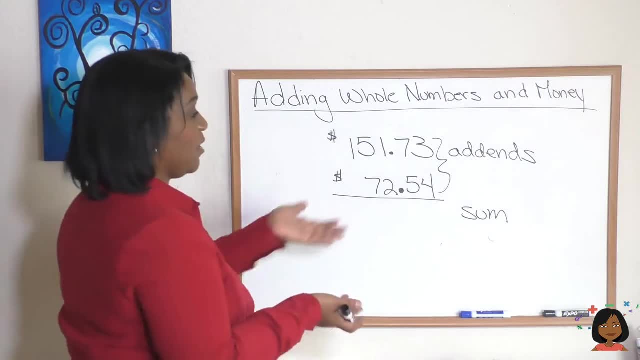 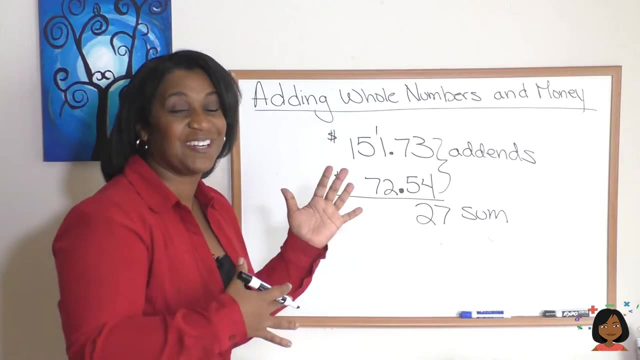 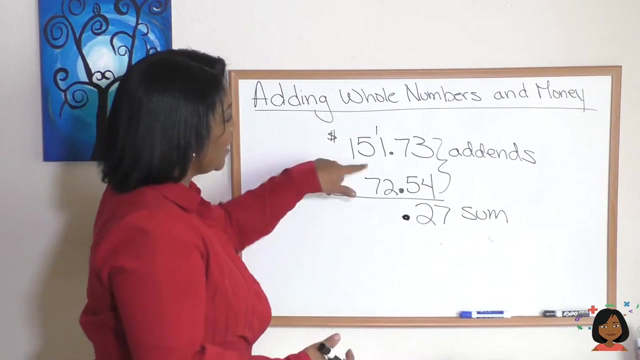 So now here I've lined up my decimal points for you so I'm ready to add 3 and 4 is 7, 7 and 5 is 12. I personally like to just bring down my decimal point right here so I don't forget that I'm dealing with money. So you can go ahead and write that decimal. Again they are lined up and keep it going. 1 plus 1 is 2, 2 plus 2 is 4, 7 and 5 is 12 and you 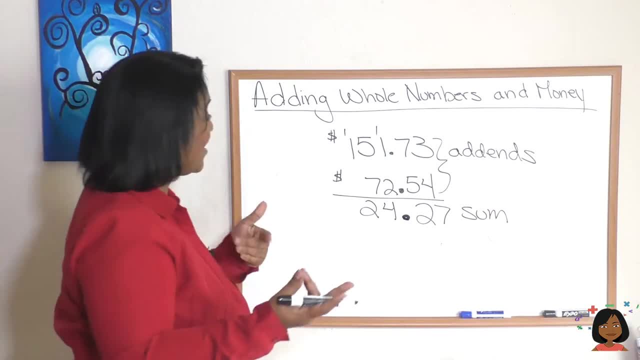 see that I've been carrying the 1 anytime I get over a number with 10. And lastly my 1 plus 1 is 2. Add my dollar sign onto the front we have 224 dollars and 27 cents. 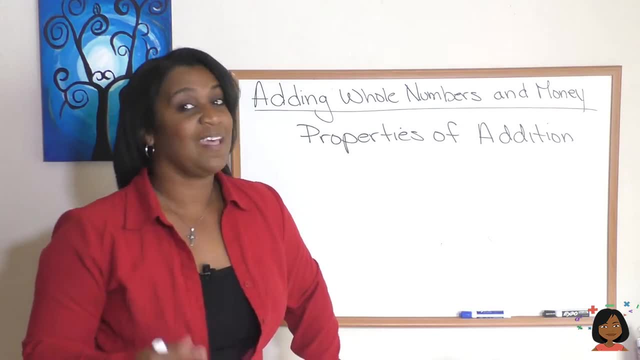 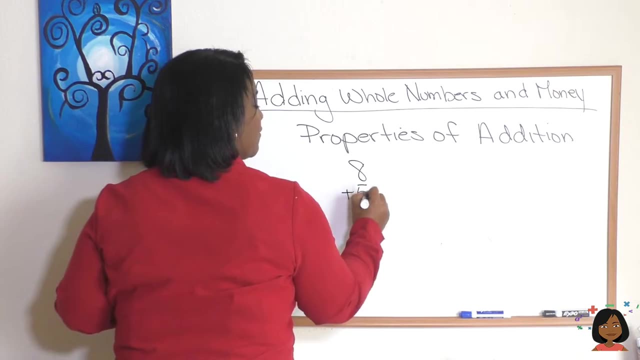 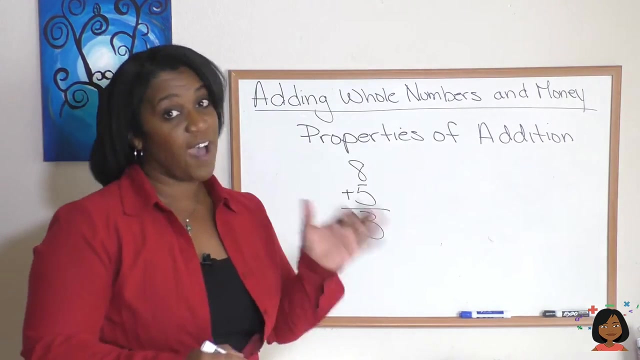 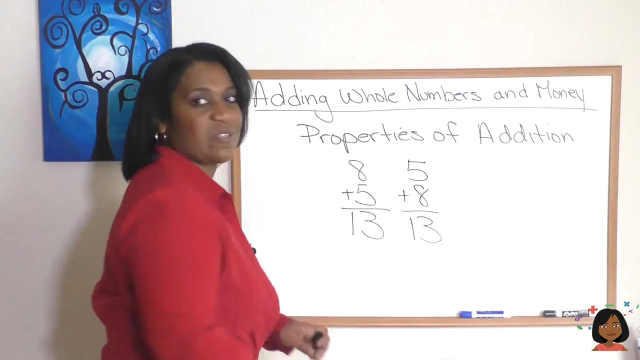 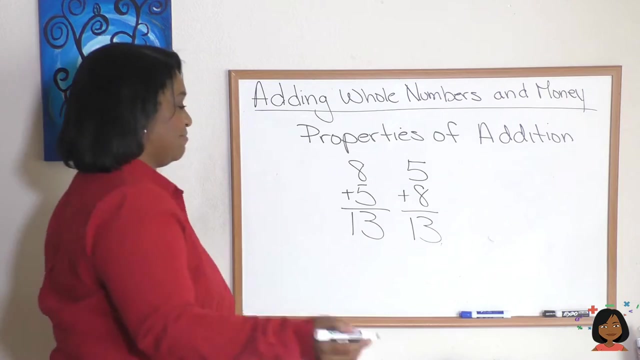 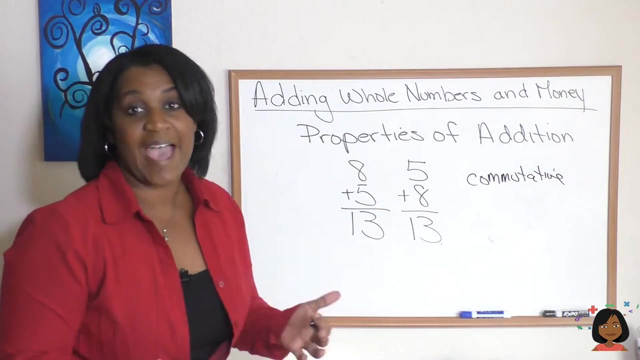 Finally I want to talk to you about two properties of addition. Take a look. So if I decided I wanted to add 8 plus 5. 8 plus 5. We know that equals 13. Okay. But what if I decided I wanted to add 5 plus 8. So I'm starting with 5 this time. And I'm adding 8. Well that also equals 13. Well in math this is a certain property that we call the commutative property of addition. Here we go. Commutative. Means it doesn't matter the order that we add the addends. The sum is still going to be the same. 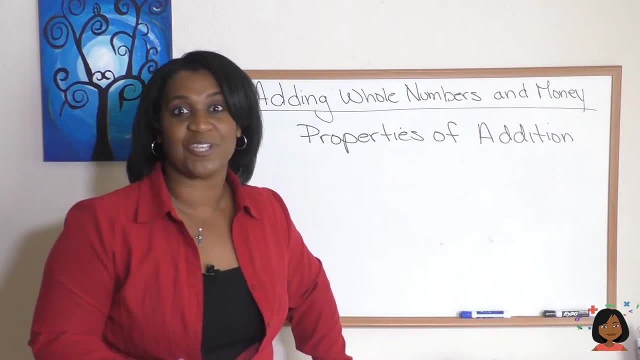 I want to introduce you to one more property of addition. Take a look. Let's say I had a number like 17. And I decided to add 0. 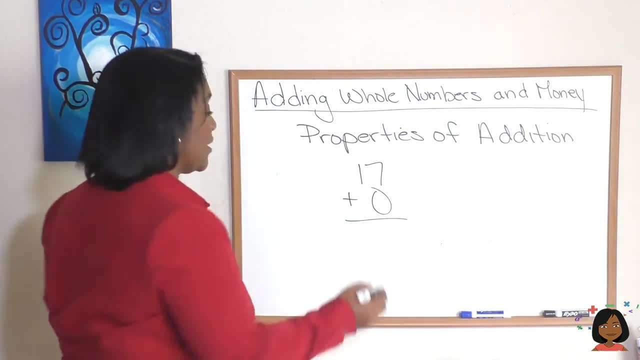 The answer is still going to be 17. 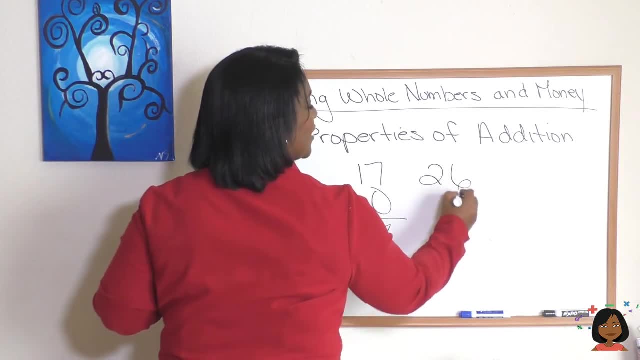 Let's see if that works for a few other numbers. If I had a number 26 and I added 0 to it. My number is still 26.